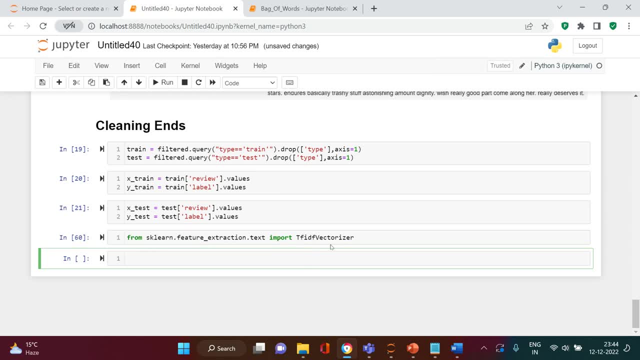 You don't need to import the transformer. okay, Now, once we are done with importing this, then we need to create the vector for it. all right, Let me call it model, I'll call it model, okay, And then I'm going to say tf, idf, vectorizer. 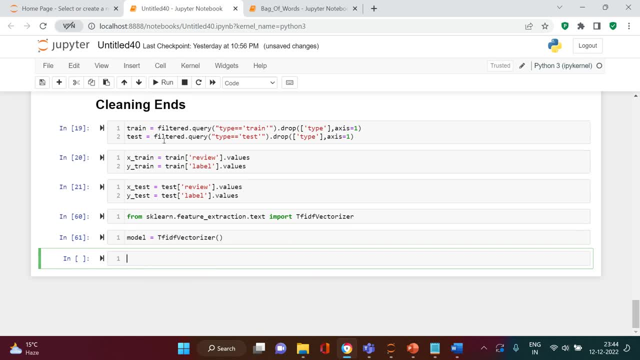 This is instance created. Now we need to, you know, train our model on this. For that we're going to say modelfit, transform, okay, And into that the data which I'm going to use is extreme. Then over here I would say: trained vector. 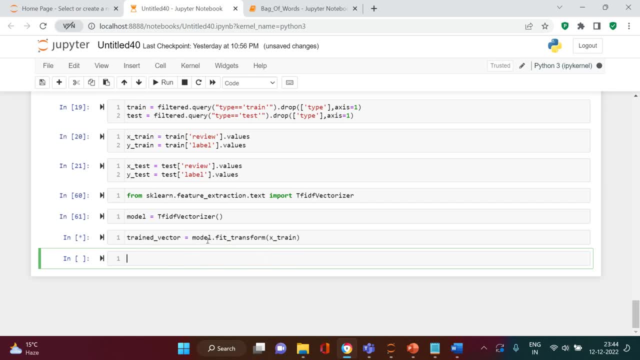 Let's call it trained vector. All right, So our vector is being trained Into here. once that is trained, then we will move forward and do the prediction. Or rather, let me call this vec, because model is something which I will be creating next. okay. 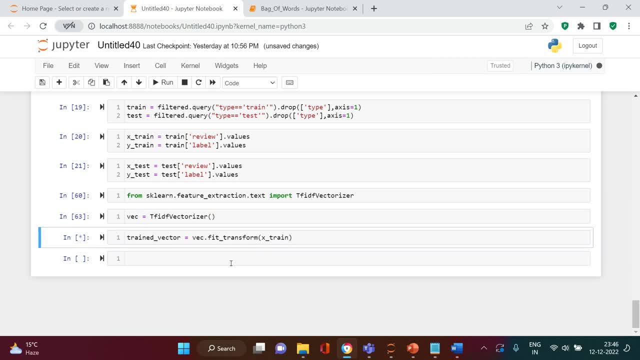 So let's just call it vec. And again, it is training, Looks like it is trained. The next thing which we're going to do is we're going to import the you know model, So I will use the naive base model over here for the sentiment analysis, same as we did. 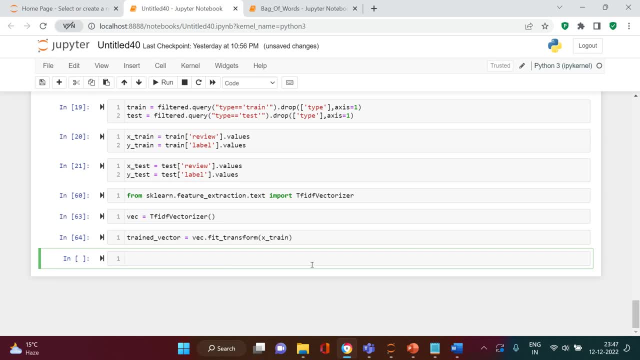 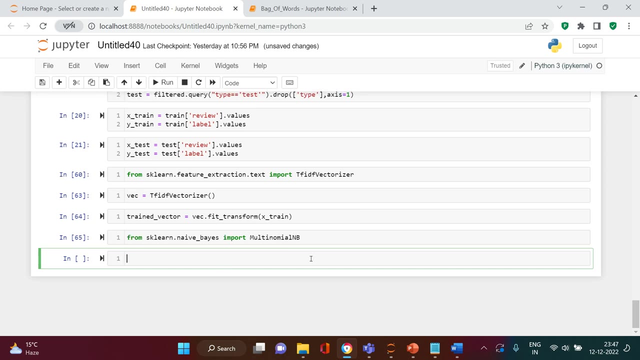 in bag of words. So how can we get that? So for that we're going to say from sklearn Let's call naive base import multinomial nb, okay. And now we're going to say model equals to multi Multinomial nb, then let's call it modelfit and inside that we're going to use the trained. 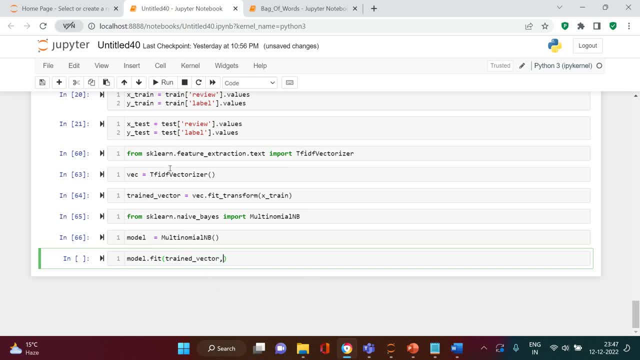 vector: Trained vector. this is the vector which we just created over here on extreme, And then we're going to say x, trained vector. And then we're going to say, y, train Right. So let's just execute. this Looks like it is done. 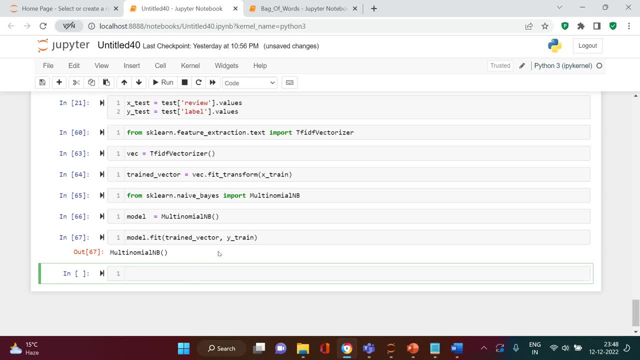 Then the next thing which we're going to- so our model is fit and okay, our model is trained. Now the next thing which we need to do is again create another vector and then then we will be using that vector for prediction. 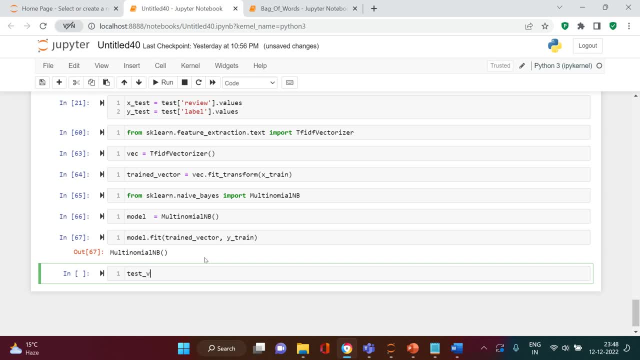 Let's do that, Okay. So for that I'm going to say test vector and over here I will say vector Check dot, fit transform and inside that I will use x test. all right, fit transform. So I will be putting the x straight data. 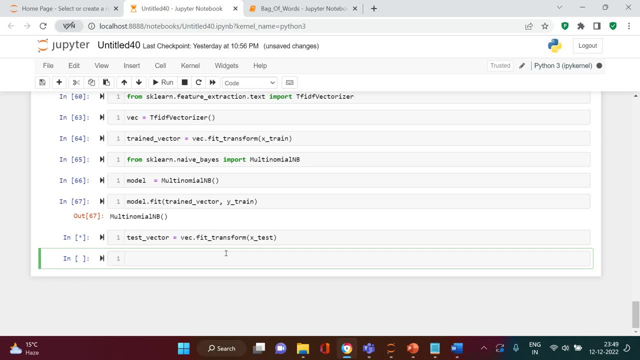 Now, once this is done, it is using just in over here. just let let's just give it few sec. All right, So this is done. Next thing which we're going to do is model which we just trained over here. 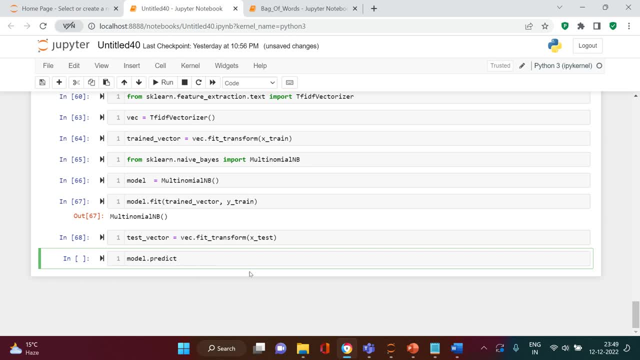 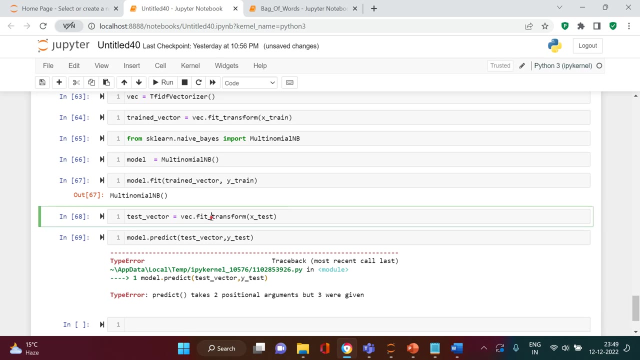 On that. I'm just going to call model dot, predict, and inside that I would say test vector, and over here I will call y, test, and let's just see: oops, predict. take two optional arguments, three were given. Let me try this and then this. let's just see if this works. 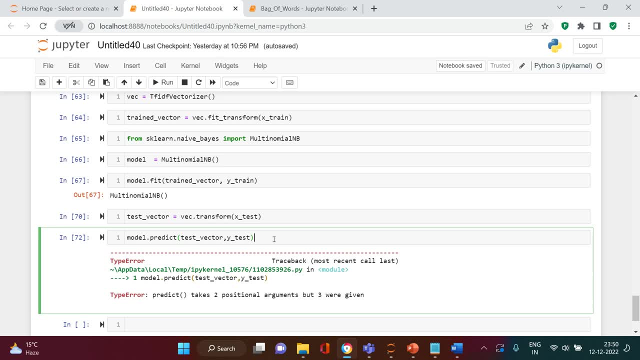 No, I just made a mistake here. I just don't need to provide this, And with this we can give it to fit, transform only, and let's just call this okay. So over here, this thing, the prediction, will be done, and then we will check the accuracy. 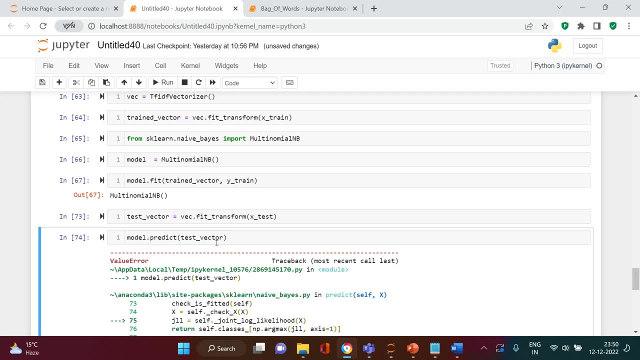 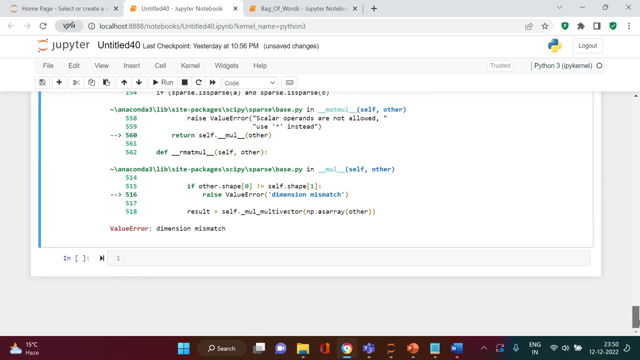 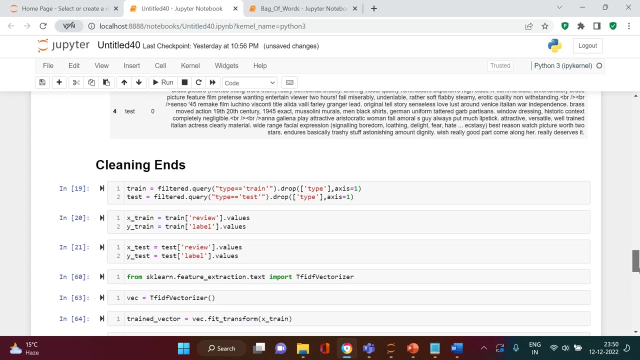 To check the accuracy, we would require to put this along with the data. Now let's see what is the problem that we got over here. Dimensions mismatch, So let's let me just do a rerun of this thing. Sometimes it just walks. 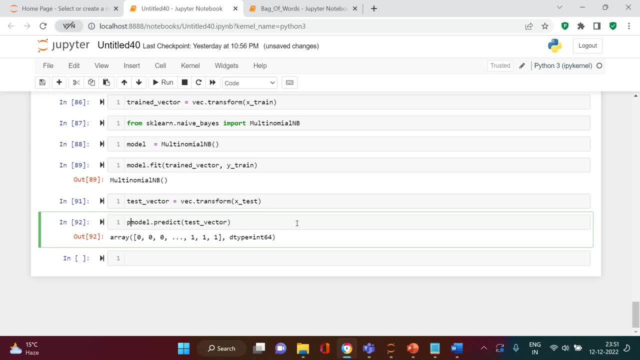 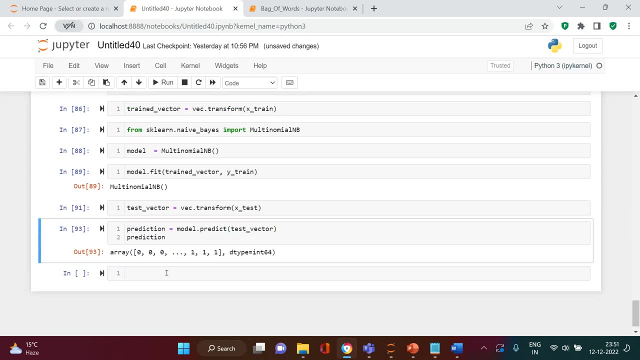 So I'll All right. So we are done with this over here. I will say prediction and let's have this prediction printed over here. Okay, Now we have the prediction, We have the X test data fit into that and now we have the y test. 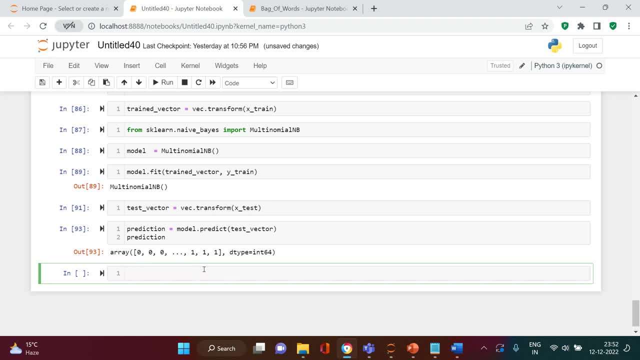 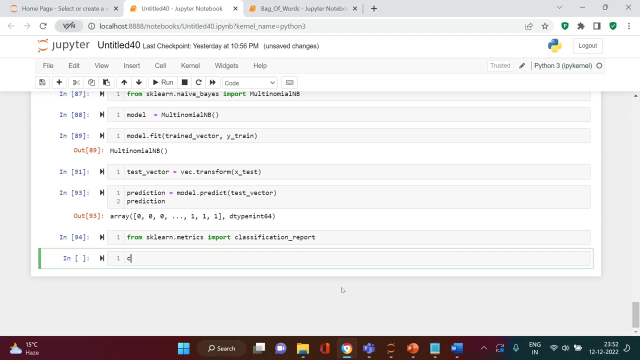 So we are just going to compare prediction and y y test value. But for that we require from sk: learn Okay. So we are going to say: prediction, dot matrix, import, import, classification report, classification report. Perfect, Now, the next thing which we're going to say is classification report. 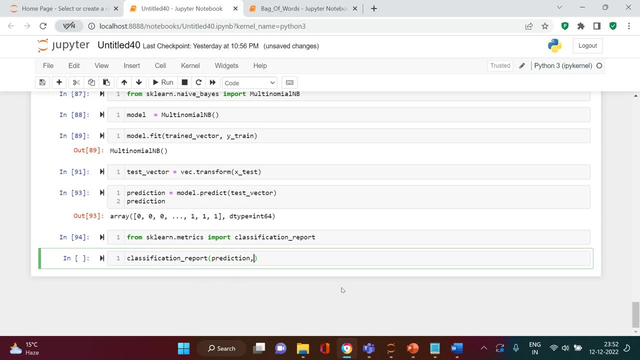 And inside that I'm going to say prediction, and then we're going to say: why test? let's run this, Okay, To make it look good. So what we're going to do is we're going to say print: oh, it's just walked. 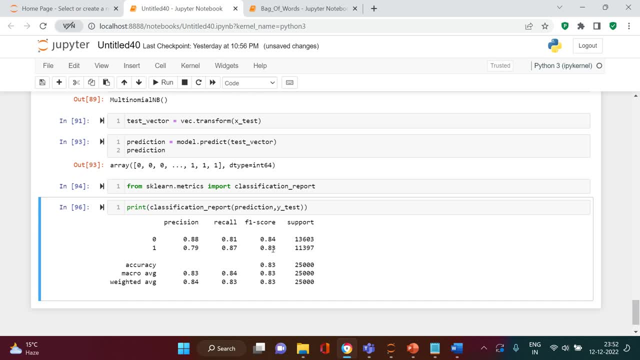 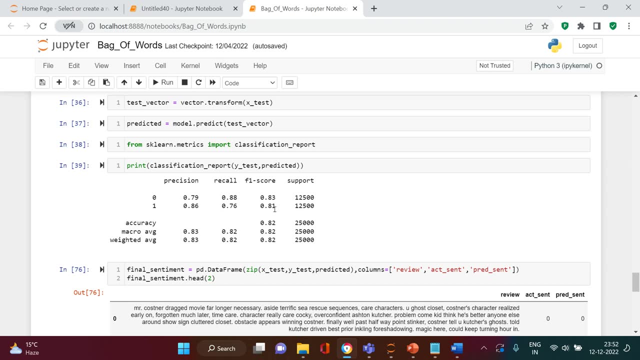 Now you see, over here, the F1 score which we got is 83%, And here which we, the F1 score which we had was just 81, right. So it is quite improvised, right? If not much, then still it's. it's better than what we had over here, right. 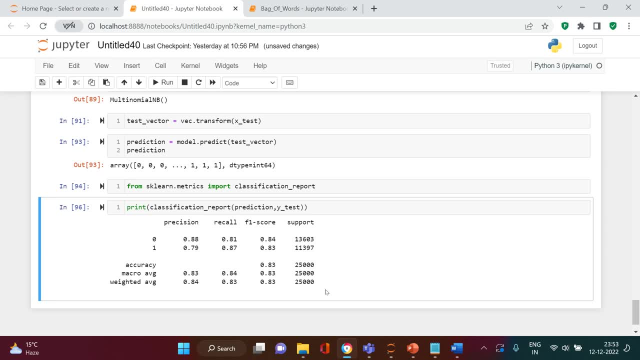 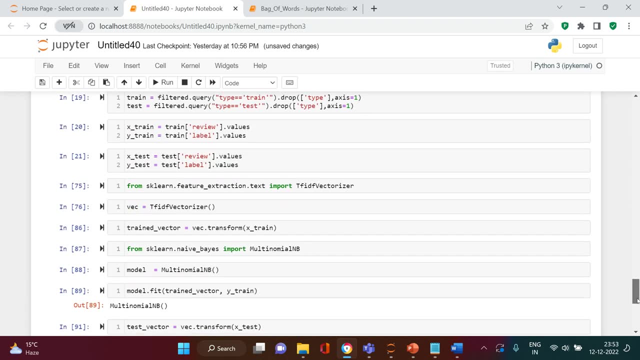 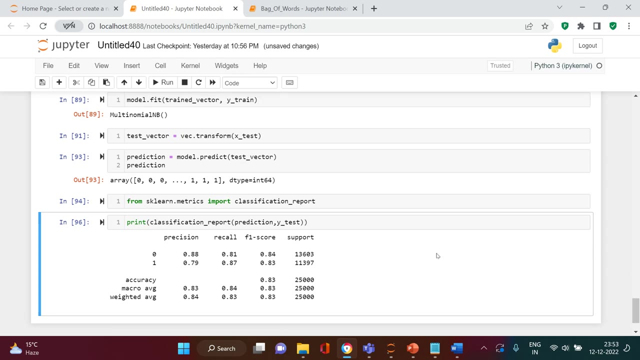 From 81 to 83.. That's, that's, that's good. I won't say it's, it's less right. So this is, this is how you can, you know, utilize the TF IDF further. If you want, you can append this prediction data into the main data frame. 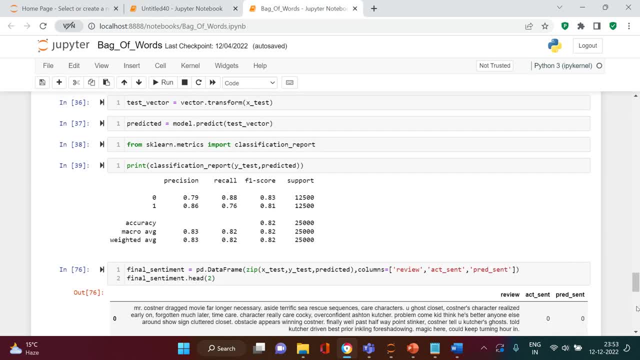 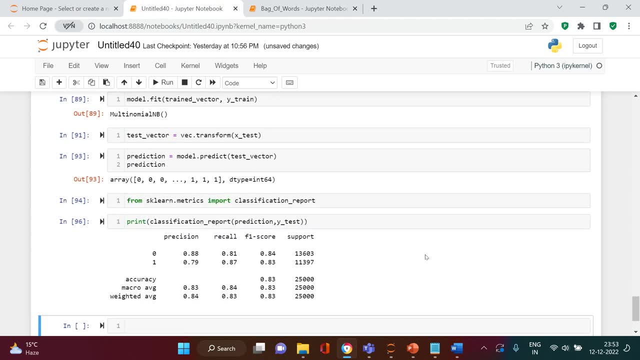 Let's just let me just do it for you. So for that, because we have the same structures, what we can do is let's just take this from here and over here. I'll simply put this: because we have the same structure, Ditto, same structure. 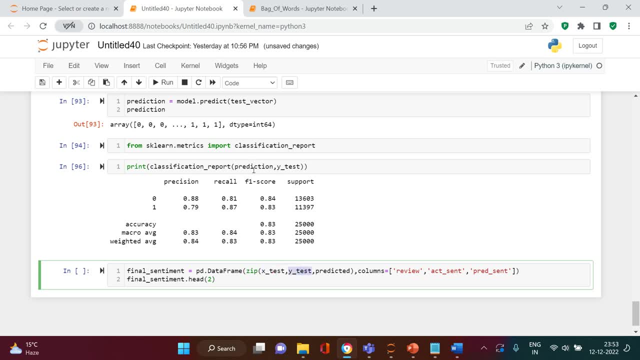 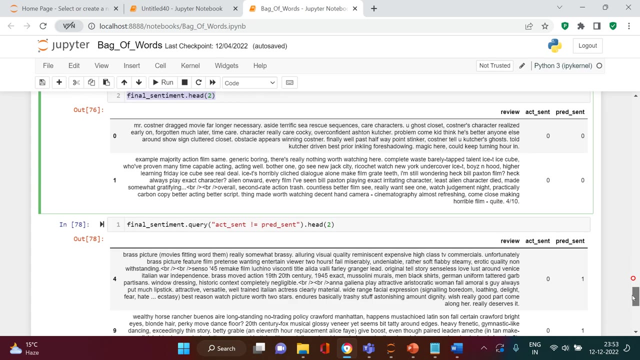 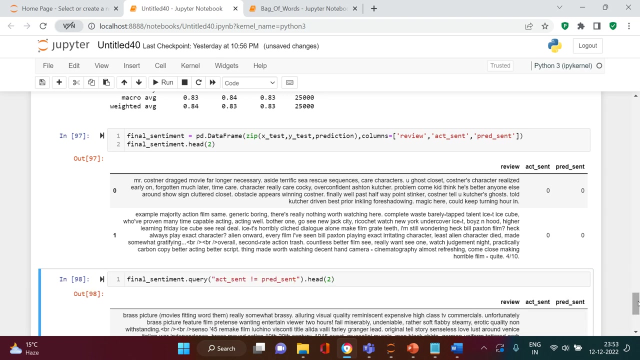 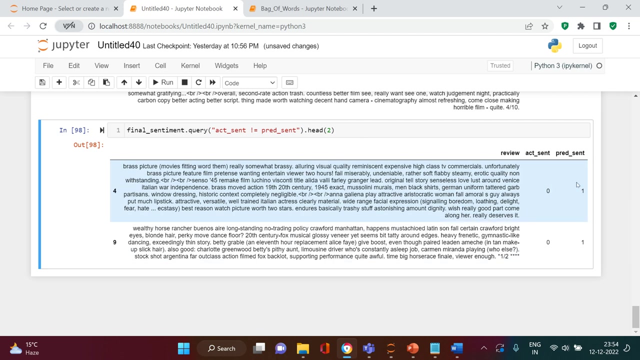 All right, Let's just run this. Oh, here, we got it. Now next thing: if you want to see where the predicted sentiment is not equals to the actual sentiment, let's try that. Here is what we got. You see over here, these are something where predicted one is not actual. 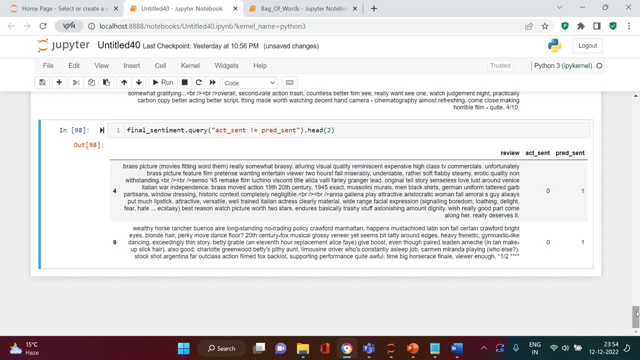 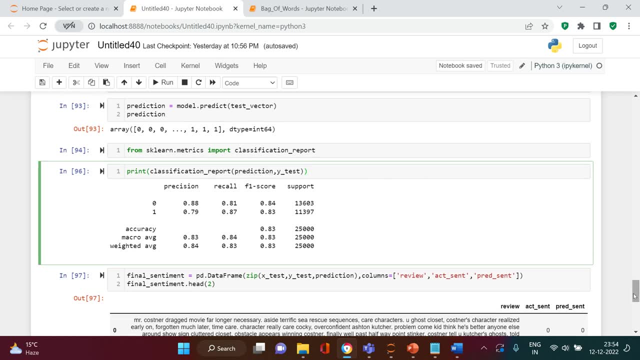 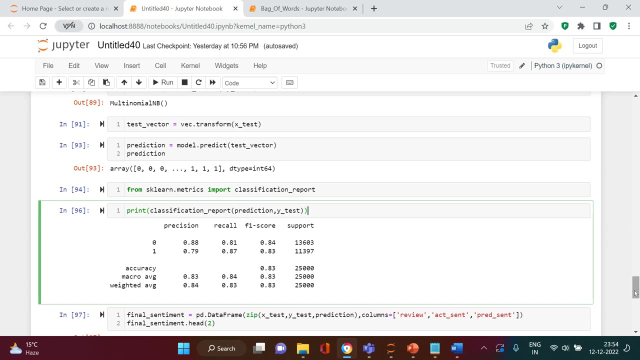 No, not equals to the actual sentiment. So this is how you can use the TF IDF. you know TF IDF vectorizer right And what TF IDF is. I explained in previous to previous video how to implement that into a, how to implement an understanding, understand it's scoring system. we, we, we- started in.